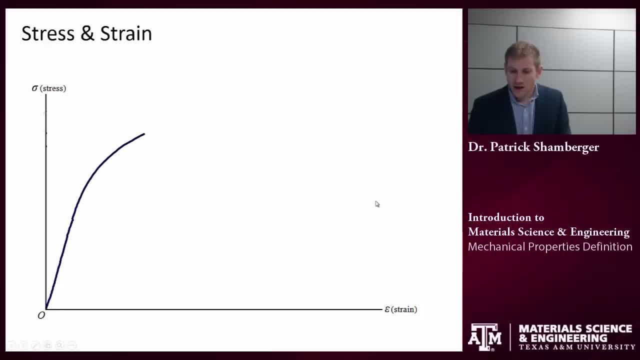 I want you to be familiar with. I'm going to draw a representative stress-strain diagram And I see that the way I drew it it looks pretty linear in here, but it starts to deviate from linearity about this point. So this is called the proportional limit, The proportional. 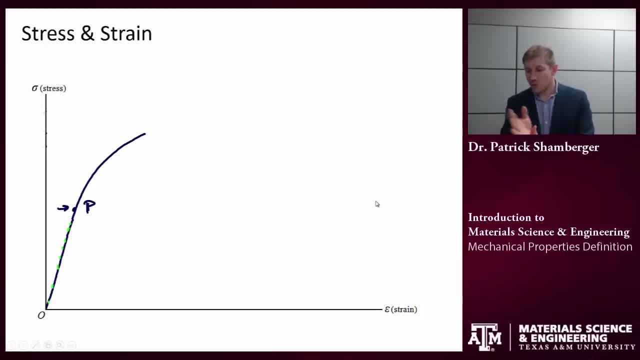 limit is divided by linearity, defined as the point at which we're no longer proportional. We're deviating from linearity. So if I was to extend that line, it would look something like that. Now, oftentimes it's very difficult. 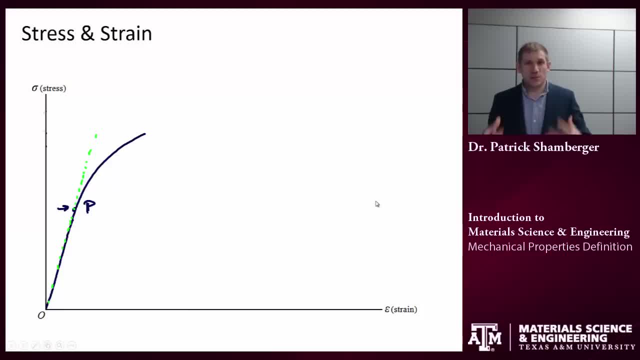 to pinpoint one distinctive stress at which this proportional limit occurs. So let me draw a second line and we'll make it a different color here. So if I was to draw a line that looked more like this- you know it's very difficult to say in there- 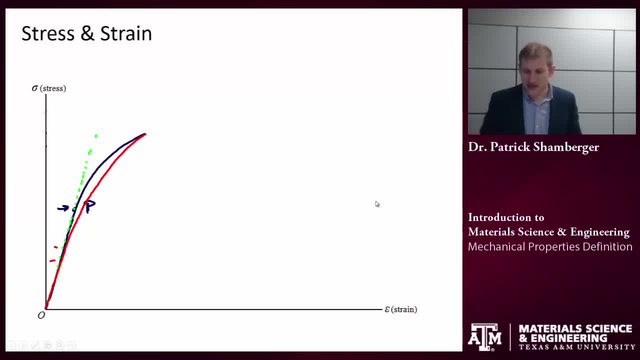 where exactly did I deviate from linearity? Was it here? was it here? So we use a convention to illustrate where we're going from elastic to plastic transformation, And the way this convention works is that we start off on the horizontal axis at 0.002 strain. 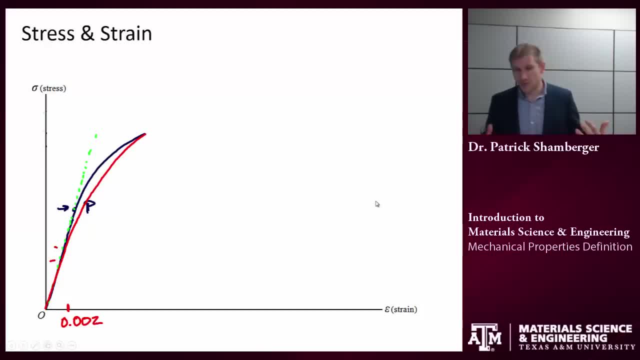 And so this is just a number that's agreed to be 0.002 strain. It's a number that's agreed upon and commonly used. Sometimes people would use other numbers, but we'll use this one, So that's the same as 0.2% strain. 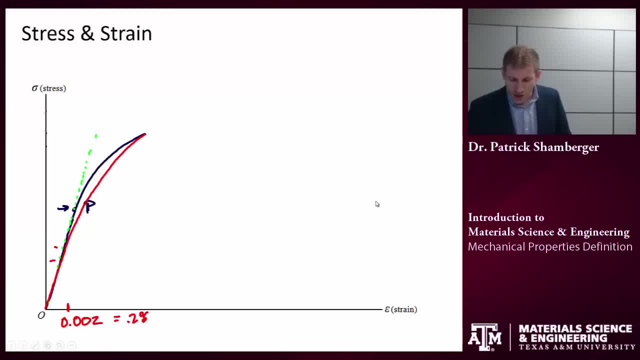 so some very small strain, And the next thing I do is I'm gonna draw a line with the same slope as this line coming out of the origin, But here I'm gonna make it a perfect line. So I could use a ruler, I could use a graphing tool. 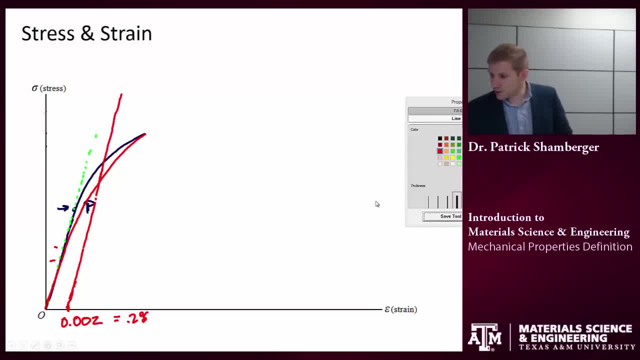 but I know that's gonna be a perfect line And at some point, at some point, these two, at some point these two lines intersect, And so this is what is commonly referred to as a yield stress, a yield point or a yield strength material. 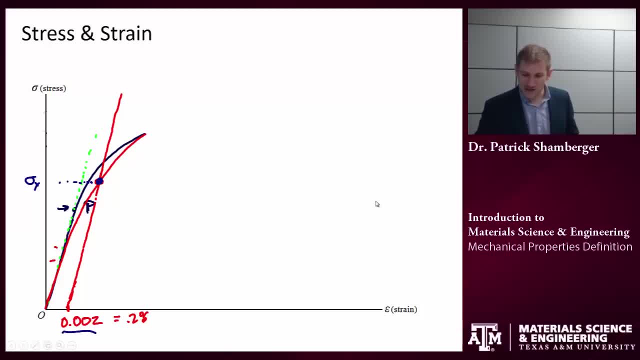 And the reason again that we use this convention is that it's very difficult sometimes to identify some specific point where it deviates from linearity. Now, that's not always true. Some stress-strain diagrams might be very distinct, and then it's easier to say yes. 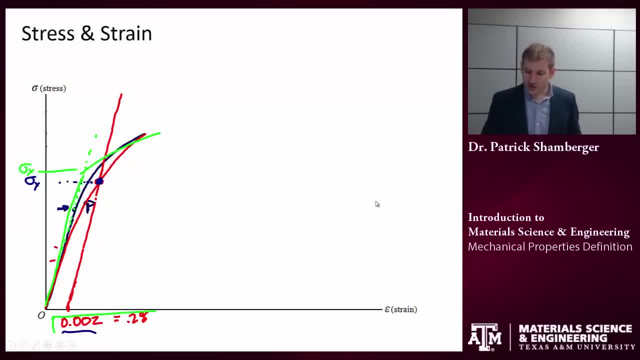 the yield stress is here, But I would encourage you to use this convention whenever possible. Okay, one other thing that you should be aware of is that certain steels exhibit a very interesting phenomenon called yield point phenomenon, And so I'm just gonna make a new axis here. 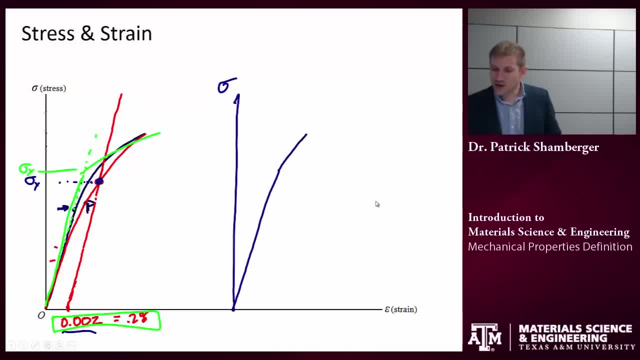 So what occurs is, again we have elastic behavior, We start to exhibit plastic deformation, but then there's a drop and there's a bit of a random stress that a material can withstand, And then it'll continue to increase and plastically deform from there. 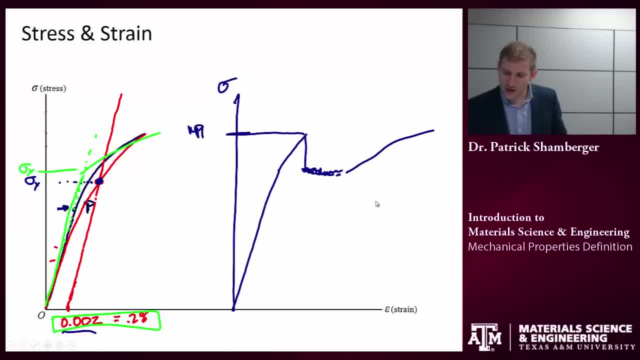 So if I see this kind of behavior, this is usually called the upper yield point Yield point And the lower yield point. And usually if I were to pick a yield stress for this material, I would pick that lower yield point, because once it goes past this upper yield point, 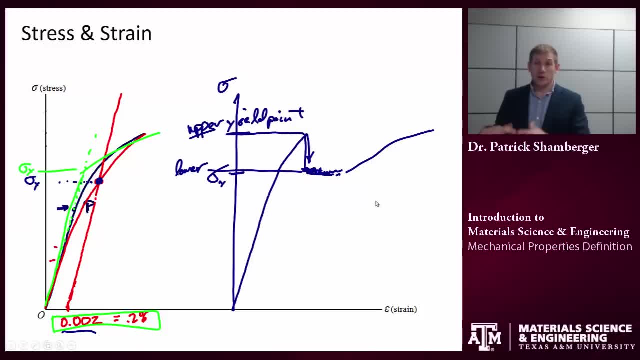 this is now the new yield stress of the material, So this is a behavior we don't see in all materials, but it's something I would like you to be familiar with. Okay, one other thing that we should think about is in this elastic region. 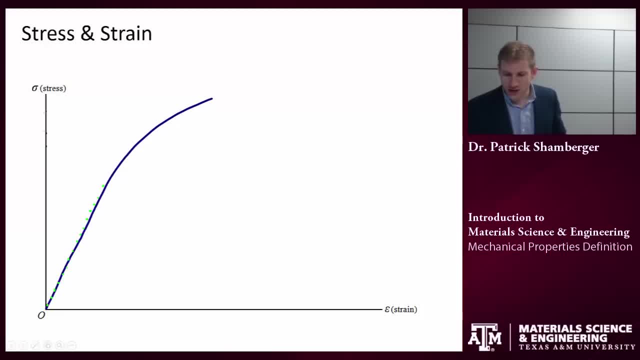 so again I have the nice linear region. here I can define what's called the elastic modulus, And this is a very specific elastic modulus. This is the Young's elastic modulus, Or sometimes it's called the tensile elastic modulus. if I'm looking at a tensile stress strain diagram. 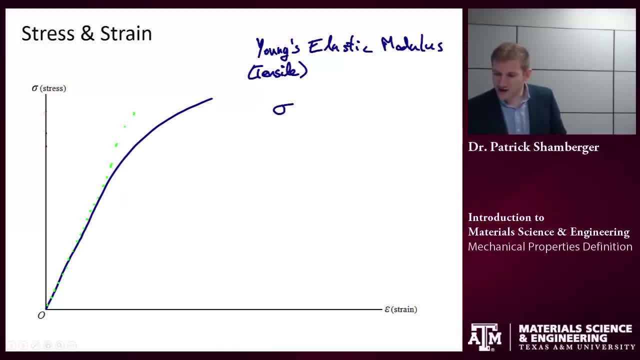 And so, because it's linear, we can describe, we can say that stress is proportional to strain And they're proportional by some constant that we call the Young's elastic modulus. And so if I were to rearrange this, I can see that the elastic modulus is just given by 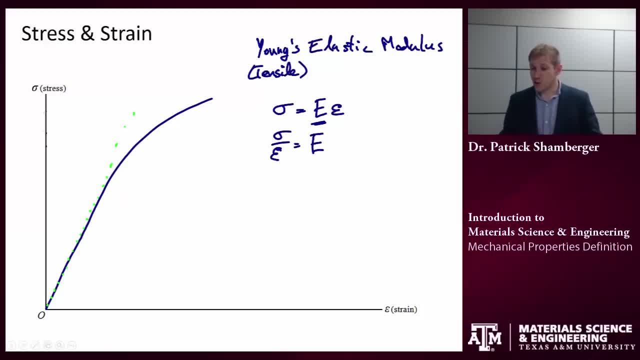 the stress over the strain, which is just a slope right. Stress is on our vertical axis, strain is on our horizontal axis, So rise over run. I can find the elastic modulus of a material just by looking at the slope of that initial linear section. 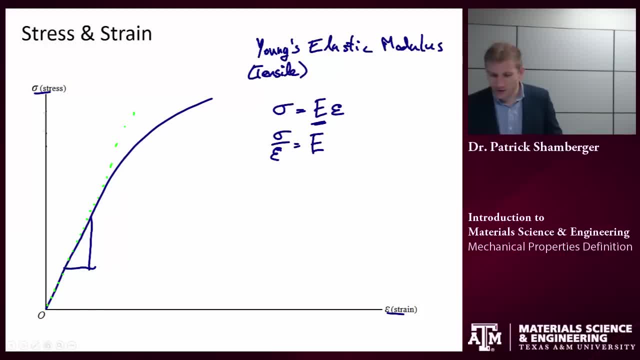 Now again, remember, materials are not always perfect, And so in some cases we might have something which is elastic, it behaves elastically, so it's totally recoverable, but it's not perfectly linear. So in this case, if I applied some stress, 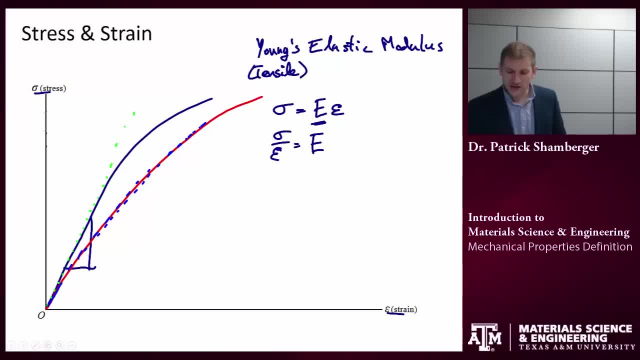 I could come up here, but I could still recover all of that strain upon removing the stress. So it's not linear. so how do we find a slope for it? There are two different things we can do. We can draw a line from: 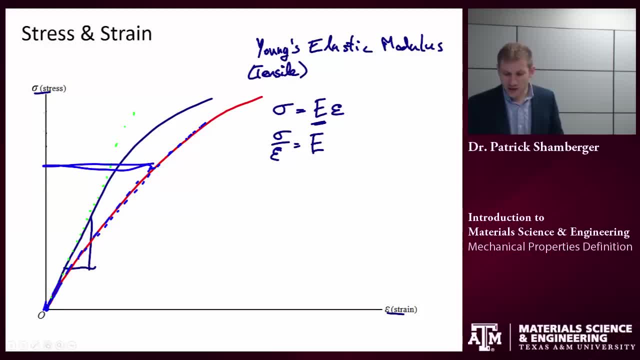 say I want the elastic modulus at this point. I could draw a line from the origin through that point, and that's what we would call the secant elastic modulus. Or I could look at the specific slope of that line at that point, And that's what I would call the. 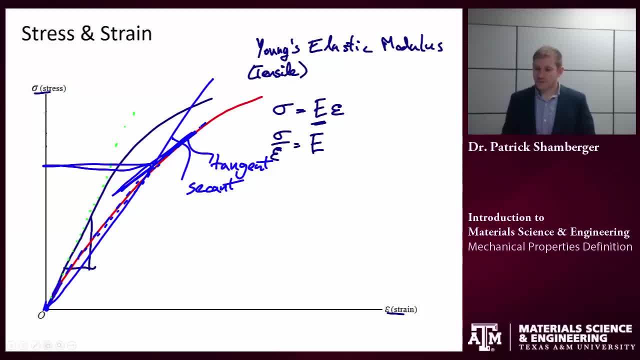 tangent elastic modulus. So again, nature isn't perfect. We try and make it perfect by our models, But these are the terminologies that you would need to know to discuss elastic behavior in materials. Okay, so we've talked about the elastic portion. 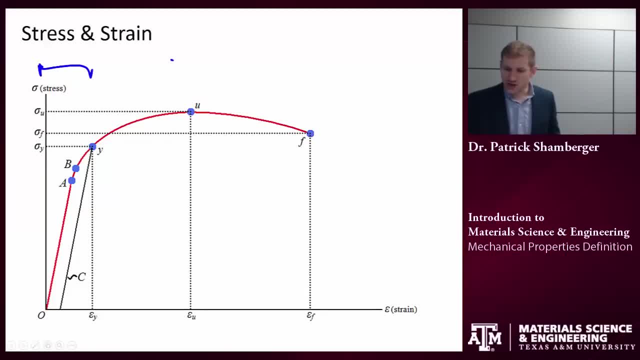 so what's going on down here? What is some terminology you might need for the other important points on this diagram? So this diagram we label here sigma sub u. This is the ultimate stress or ultimate strength of a material. I should mention that this is kind of a typical curve. 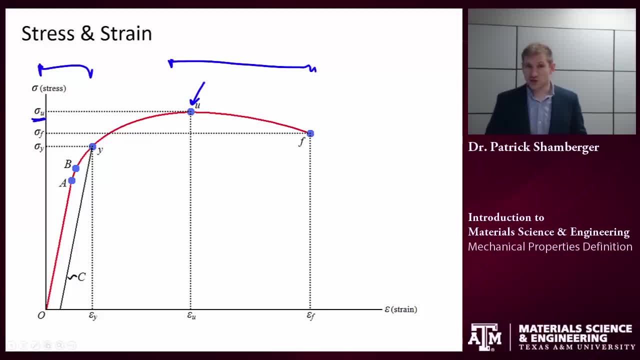 for metal that we're looking at. So usually this point is associated with necking- And we'll talk about necking at some future point. But this is called the ultimate stress, That's the maximum of the stress-strain curve. And finally, this is called the failure point. 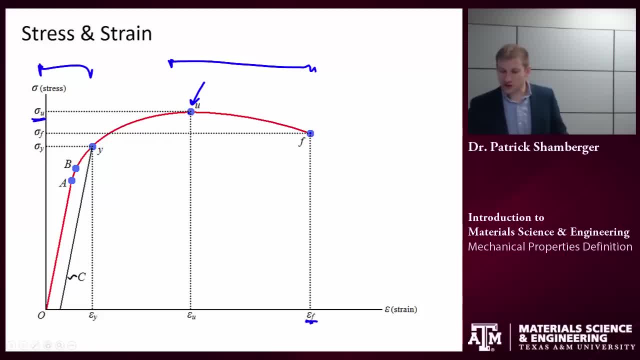 The failure stress, failure strength. This would be the failure strain point, And this is when the material actually breaks entirely on you. So this is a very important point in terms of what's happening under extreme plastic deformation, One thing that we often talk about in materials. 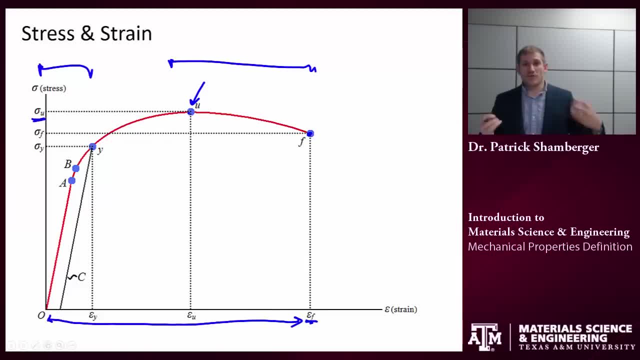 is their ductility, How much can they deform before they break? And so one measure of ductility is the percent elongation at failure, And that is exactly what the failure strain is. So a percent elongation would be delta L over L times 100.. 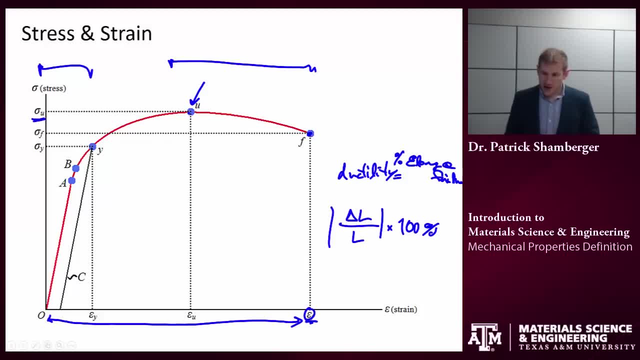 And strain again. remember is just delta L over L, So that is ductility. One other thing that I wanted to talk about. I guess we're using the same graph. We can talk about how much energy it takes to either break a material. 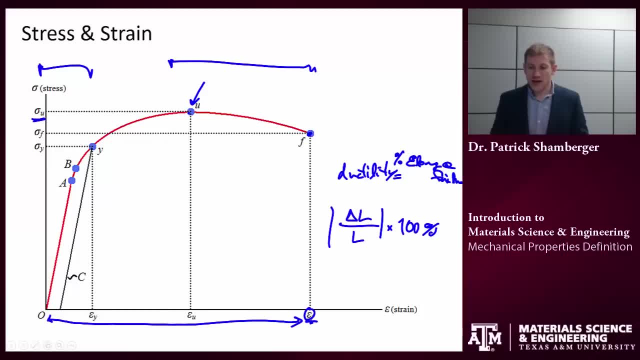 or how much energy can be stored elastically, And how we do that is by integrating different areas of the stress-strain diagram. So if I were to integrate the stress-strain curve from integrate stress-destrain, from zero to the yield point, 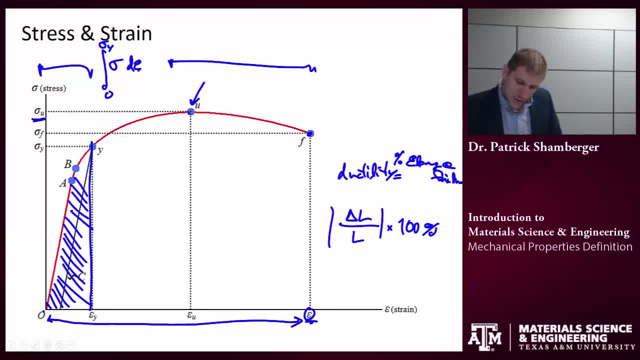 I would get this area here, And this is usually called the modulus of resilience, And so this tells us how much energy can a material store elastically If I were to integrate the entire area under the curve, so from zero up to the failure. 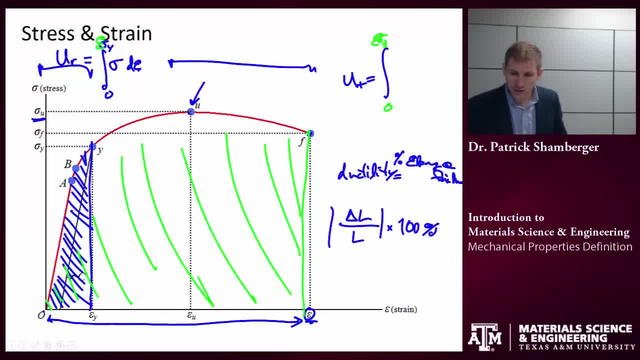 sorry, this should be: strain up to the failure. strain again stress-destrain, if I get the area under that whole curve, that's a measure of how much energy it takes to break the material. Now this would be a kind of a static measure. 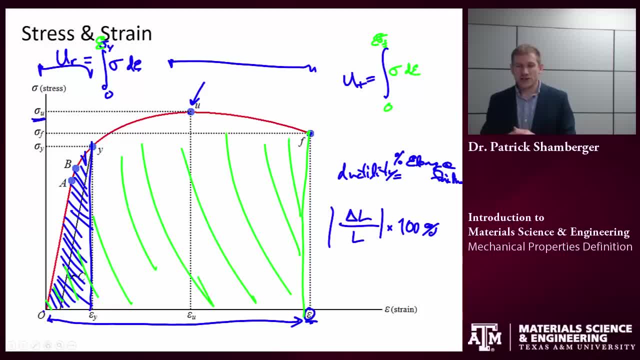 of that, because these are usually captured by deforming a material very slowly. There are other ways to measure this toughness, So this is the modulus of toughness. There are other ways to measure the toughness by a more dynamic experiment, So essentially swinging down a heavy weight.